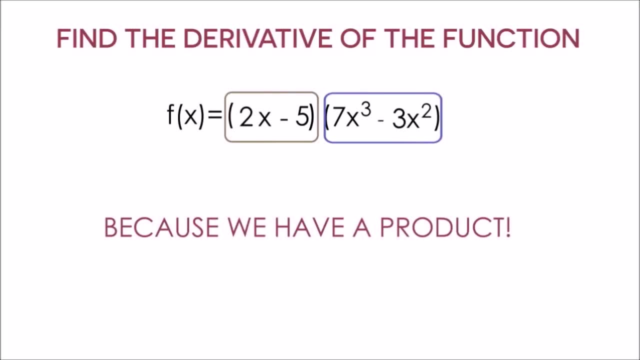 Anytime we have two things being multiplied with each other, we have to use the product rule to take the derivative And notice how we do have two things being multiplied with each other. We have the 2x minus 5 being multiplied with the 7x cubed minus 3x squared. So let's use the product. 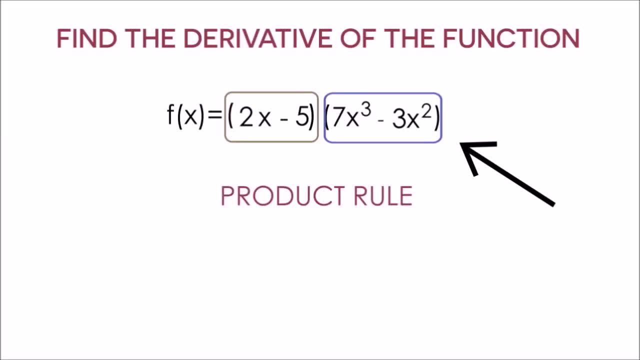 rule to take the derivative of this function. So the first thing I like to do is to label our two things being multiplied with each other. So I'm going to label the 2x minus 5 our first thing, and the 7x cubed minus 3x squared I'll label as our second thing being multiplied. 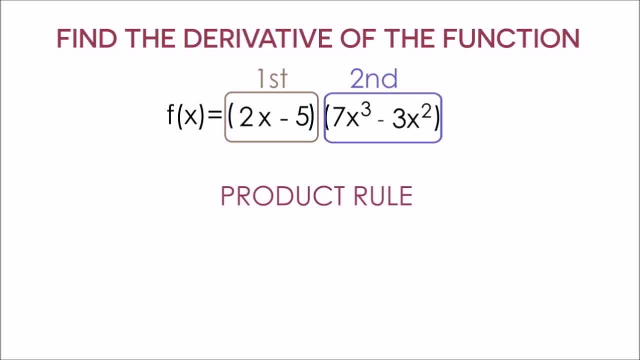 And now we can use the product rule formula to take the derivative of this function, And the product rule formula is the first thing multiplied times the derivative of the second, plus the derivative of the first, multiplied times the second, And the only thing we have to do is plug. 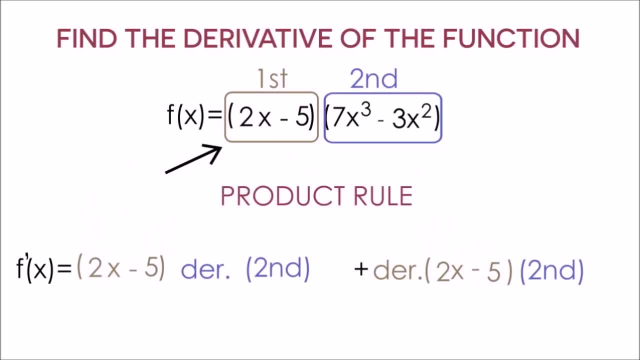 in our first thing of 2x minus 5, everywhere we see first, And we can plug in our second thing of 7x cubed minus 3x squared. And we can plug in our second thing of 7x cubed minus 3x squared. 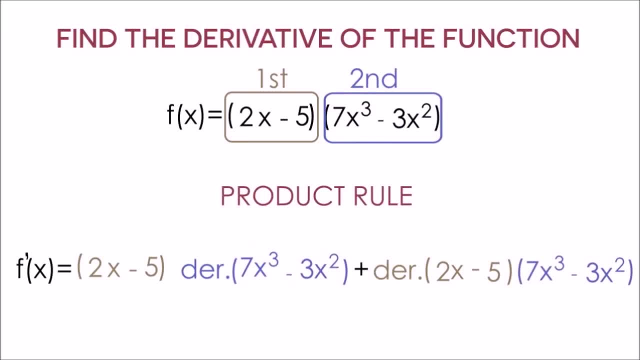 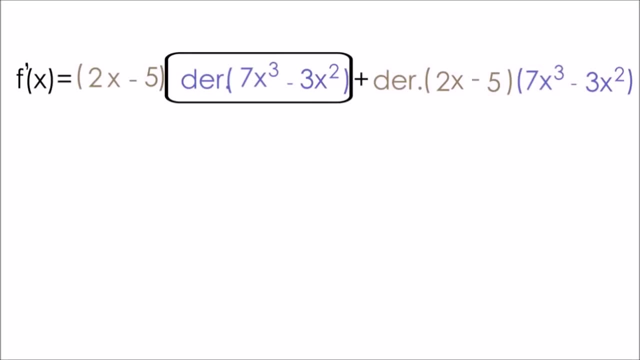 And we canاض plug in our second thing of 7x squared every time we see second. All right, So now I need to simplify this as much as part possible. So I'll start start by taking the derivative of 7x cubed minus 3x squared, and the derivative of 7x cubed is 21x2 and the derivative of 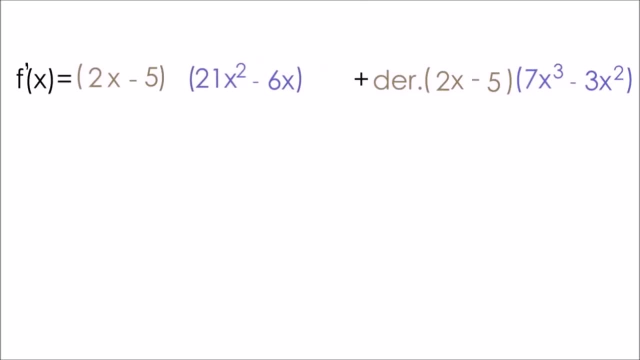 negative 3x squared is equal to negative 6x, And if we move to the right, we can take the derivative of 2x minus 5.. The derivative of 2x is just 2, the. the derivative of negative five is equal to zero. 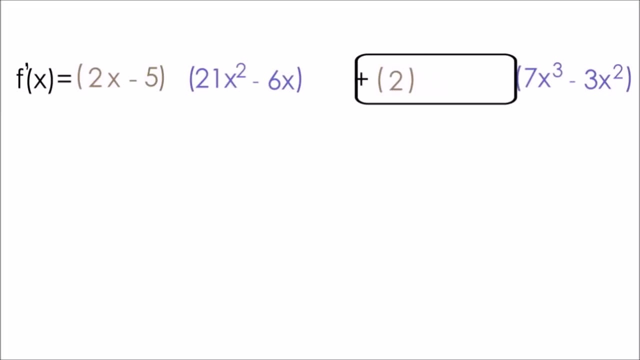 So this just simplifies to two. All right, so now we have to do a little bit of algebra to simplify this even further. The first thing I'll do is distribute the two x minus five with the 21 x squared minus six x. 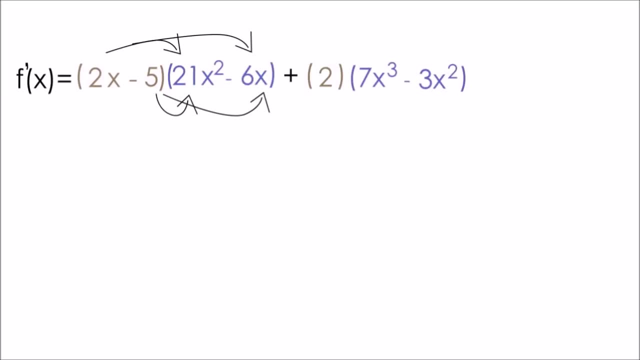 If we FOIL and multiply all of these terms together, we get 42 x cubed minus 12 x squared minus 105 x squared plus 30 x. And if we keep moving to the right, we can multiply the two with the seven x cubed.